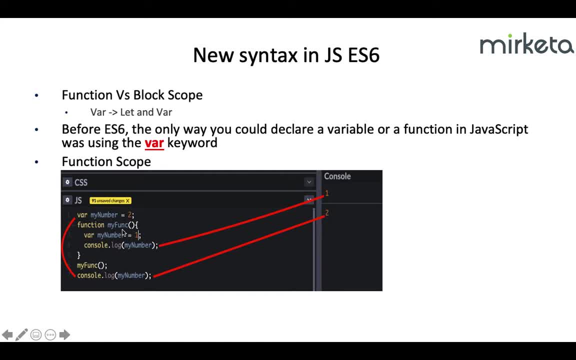 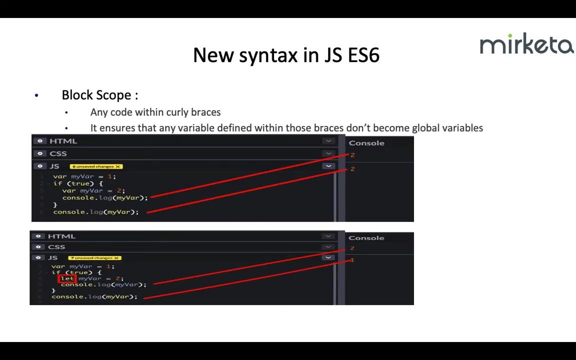 see the code. we declare var with same name in global context and within the function. So, as expected, we can see the var within function. We can see the values as two for the global context and one for the function scope. Everything works great, right. 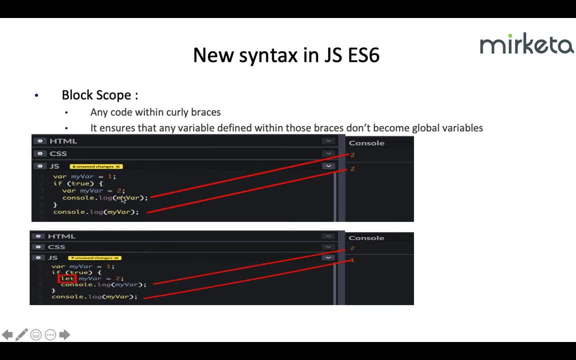 If you see the below code, code year. we declare a variable, my var, same as a global variable And we declare var in the same way. So we declare var in the same way And we declare var in the same way. 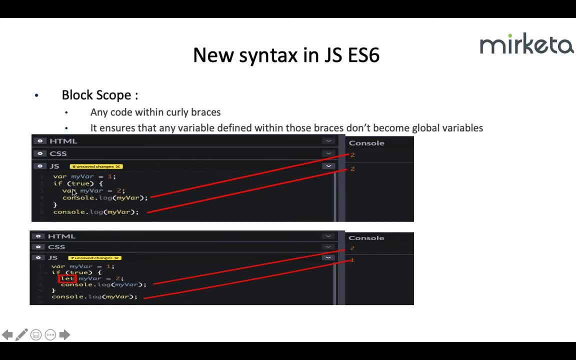 And we declare var in the same way, And we declare var in the same way. So here and here the output, what we got is not as expected. Here you can understand what is block. A block is any code within curly braces. Block scoping ensures that any variable defined within those braces don't become global variables. 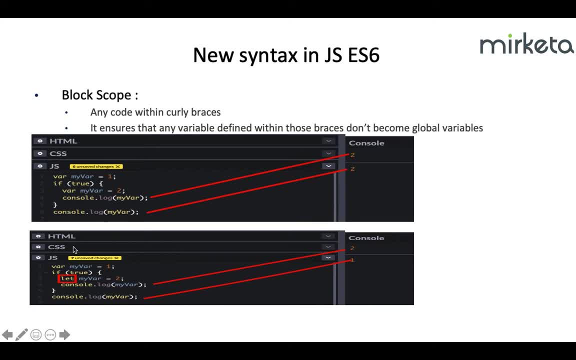 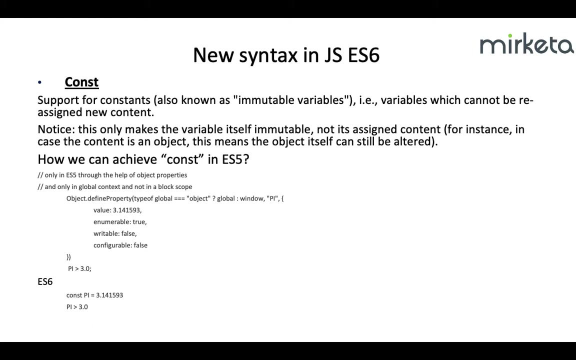 Here, ES6 introduced let, which holds values within the scope. If you see this code, the values looks good. So values: two for this within the block scope, one for the global variable. Okay, next one is the constant. So what is constant? It is a. 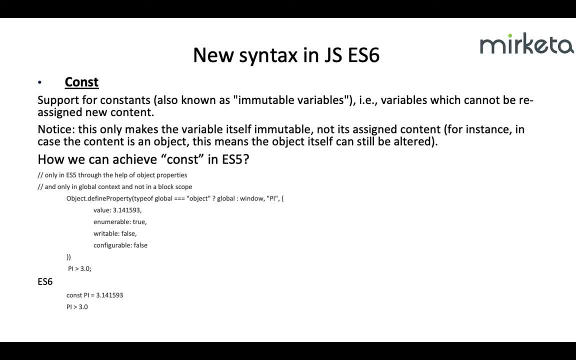 variable which cannot be reassigned. new content. If you see the code year, how we achieve constant in ES5.. Lot of code, right So, but we can achieve same with one line of code in ES6.. Okay, here is the note. we make the variable itself immutable, not its ascent content. This means the object. 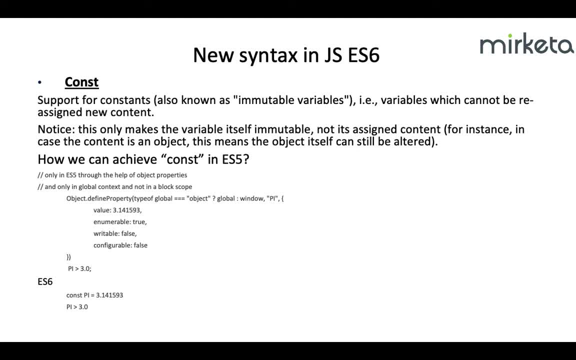 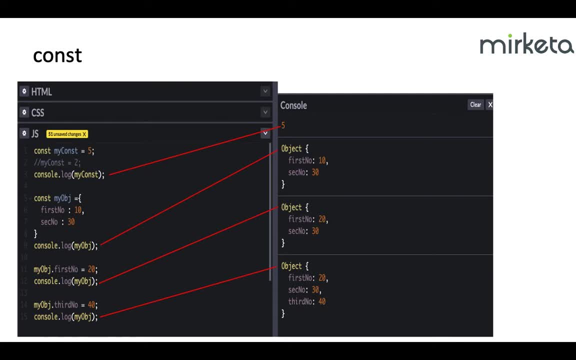 itself can still be altered. It is the code. sorry, It is the code, Okay. first, if you see, the first line assigned a constant variable, s5, and I try to change the value to 2. it threw me some error, that's why I just comment it out. so if you see that below code I: 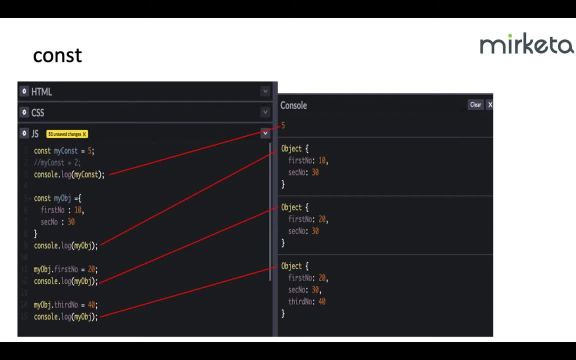 create an object, I introduce two properties and then in line number 11, I alter the first property and also in the line number 14, I introduce in your property. so everything works expected. okay, this means that it is possible to change the value to 1 and I try to set it to 12 and it will be. 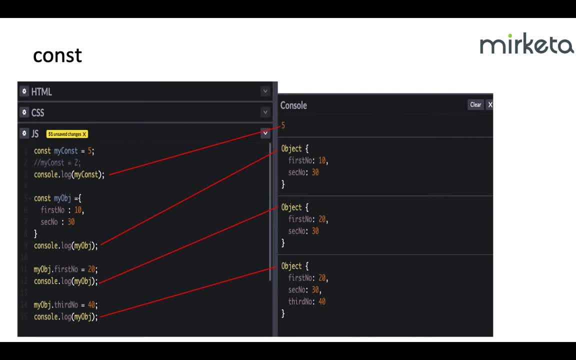 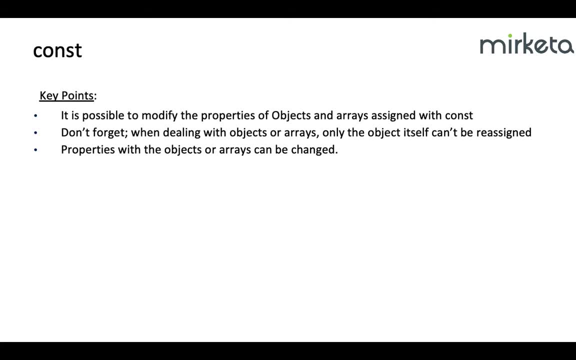 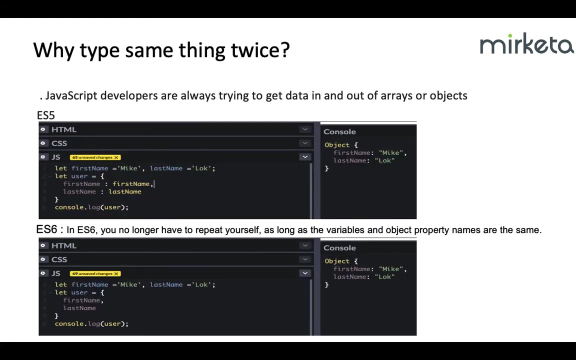 to modify the properties of object and arrays assigned with constant right. so these are the key points, don't forget when dealing with objects or arrays, only the object itself cannot be changed. properties within the object or arrays can still be changed. okay, next point is assigning the properties. if you see, 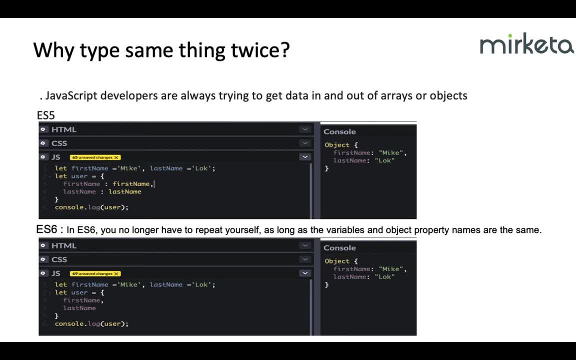 that. so we always trying to get in and out of arrays and objects. so whenever we assign some properties within object, so for example, first thing we declare some variable here and use the same variable in that object, right? so here we declare first name and last name and we assign the same thing. 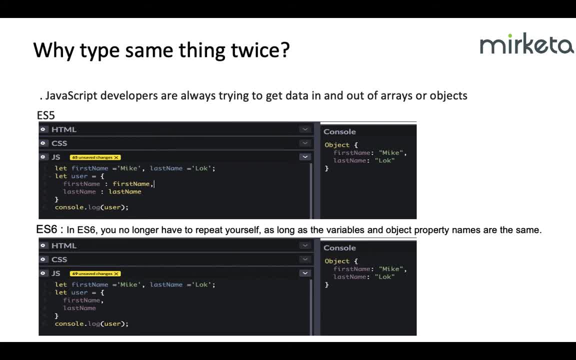 in the user object, but in ES6, if you try to use the same name, then there is no need to type it twice. if you see the code below here, instead of writing first name two times here you can declare it only once and it will take it. 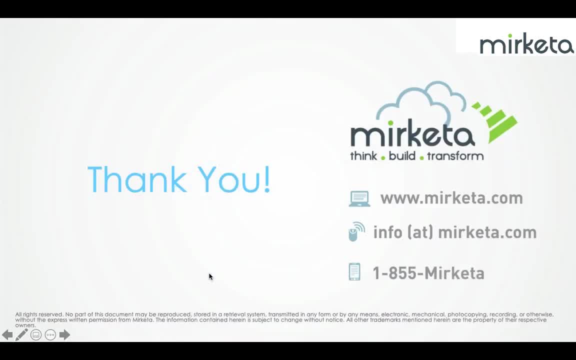 up. okay, that's all from today.